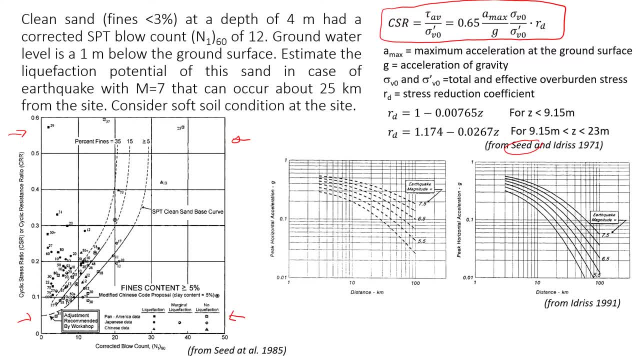 not. So let's look at this example that is written here. Let's say that we have a clean sand, which means that we have fines less than five percent- in this case, less than three percent- at depths of four meters and when SPT test was performed and correlated to the energy of hammer. 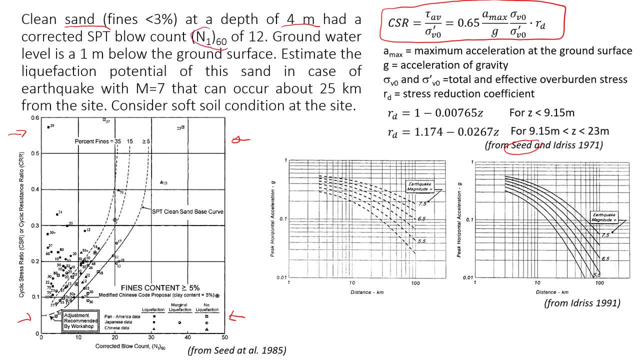 and to the overburden pressure. this N160 was 12.. Also, During site investigation, it was found that the groundwater level was one meter below the ground surface, so it was pretty high And let's estimate the liquefaction potential of this sand in case of there is an earthquake with magnitude of seven. 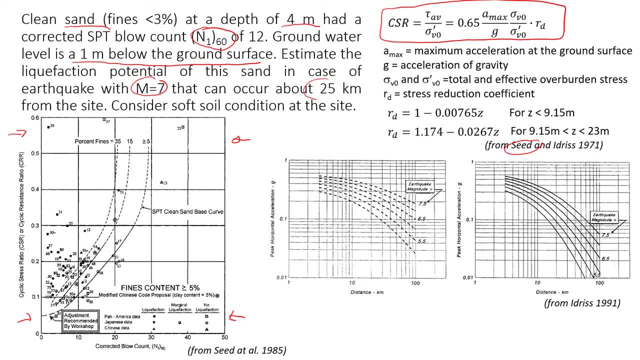 And the epicenter will be about 25 kilometers away from the investigation site, And also we should consider soft conditions at the site, And I will explain why we need this one. Okay, so to do that, we're going to use this procedure to calculate cyclic stress ratio. 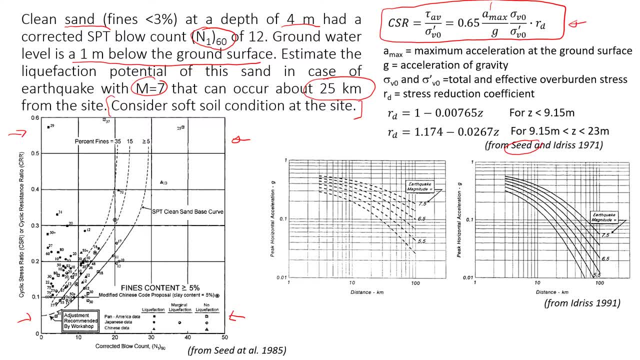 You will see that what we need to know is peak acceleration at the surface, And we need to know the effect of vertical stress here, this one, and total stress as well. And there is this coefficient- it's called stress reduction coefficient- We can roughly estimate. 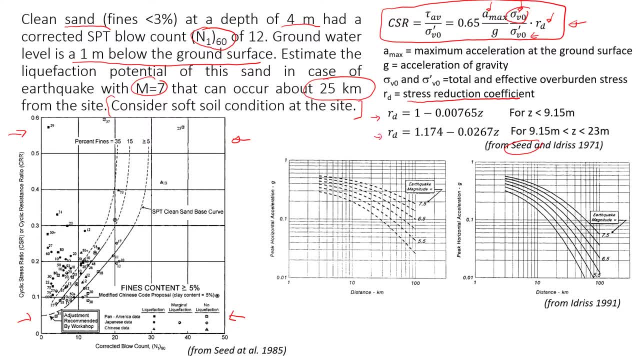 It's using these two empirical formulas, So this one for the depth less than 9.15 meters And this one will be for the depth that is greater than 9.15 meters but less than 23 meters. So you will see that in our case the depth is four meters. 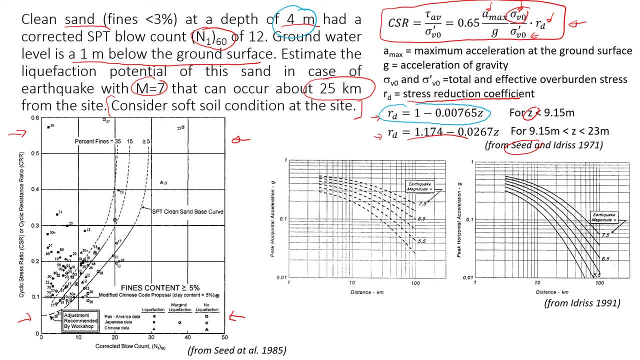 This means that we're going to use this value of stress reduction coefficient. Okay, now let's find it, I'm going, I'm going to write it down here. So this coefficient will be equal 1 minus 0.00765 times four meters. 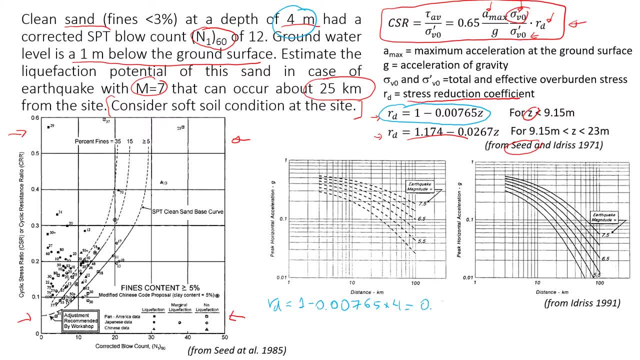 So that will give us approximately 0.969.. Okay, so we found this. Now we're going to find maximum peak acceleration at the surface. To do that we're going to look at these two charts proposed by Idris in his work in 1991.. 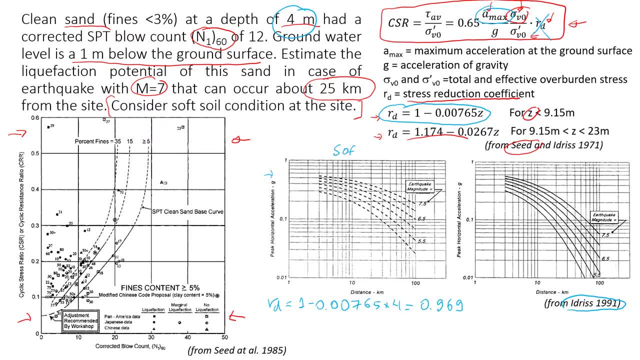 So this one is for soft side conditions and this one is for what's it called rock side conditions. So in our case, we have soft conditions, So we're going to use this chart. So in this case, we're going to look at the distance to the epicenter. 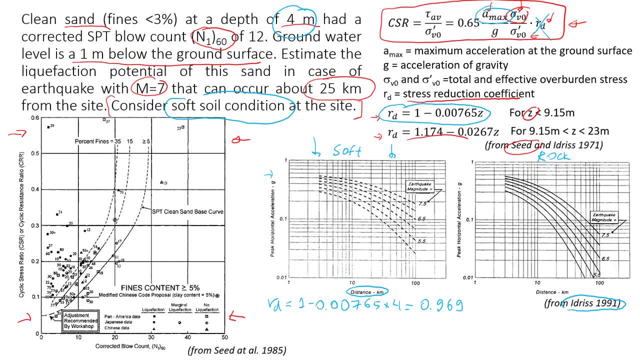 And in our case it's 25 meters, 25 kilometers here, and magnitude is 7.. So it will be about here. So you will see that this point, that will be about 0.3, 0.3 g. 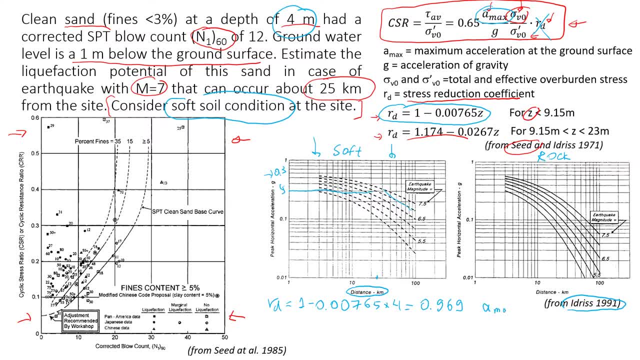 So we're going to write that maximum acceleration that can be expected is 0.3 g. Next step is total vertical stress. So to find total vertical stress we need to find the unit weight and multiply it by the depth. So we don't know. the unit weight of descent is not given. 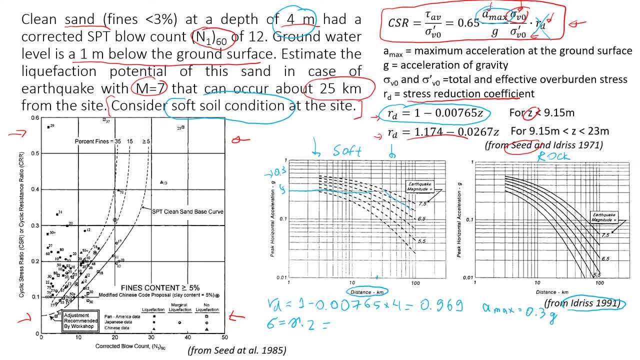 So we'll assume that common unit weight is 18 kilometers per square meters. 18 times four will give us 72 kPa. So now we need to find the water pressure. For the pressure, it says that it's one meter below the ground and we have four meters to the sand of interest. 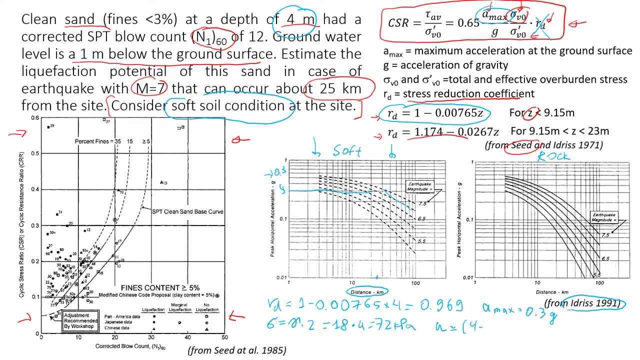 So in this case it will be four minus one meters, times the unit weight of water: 9.81.. So that will give us 29.43 kPa. And now let's find the vertical effective stress. So it will be total stress minus power to pressure: 72 minus 29.43.. 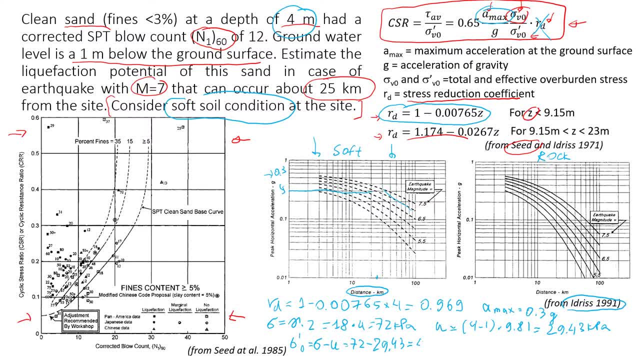 That will give us approximately 42.6 kPa. Okay, so now we're going to estimate cyclic stress Ratio. I'm going to raise this one, So we're going to write now that cyclic stress ratio. Cyclic stress ratio. 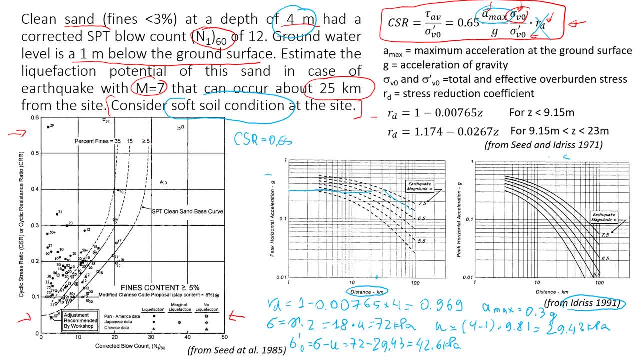 It's 0.65 times the peak acceleration, which we decide is going to be 0.65.. So 0.3g divided by g. So in this case, same thing. Then multiply by the total vertical stress, which is 72,, divided by effective vertical stress: 42.6.. 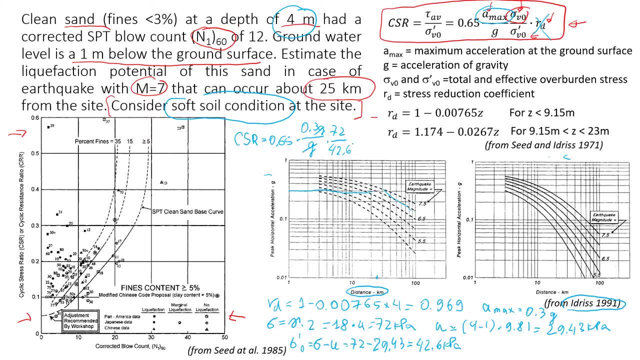 And times the stress reduction coefficient, which is 0.969.. So according to my calculations, we're going to get about 0.319.. So this is the value. So now let's look at this chart And here it says cyclic stress ratio. 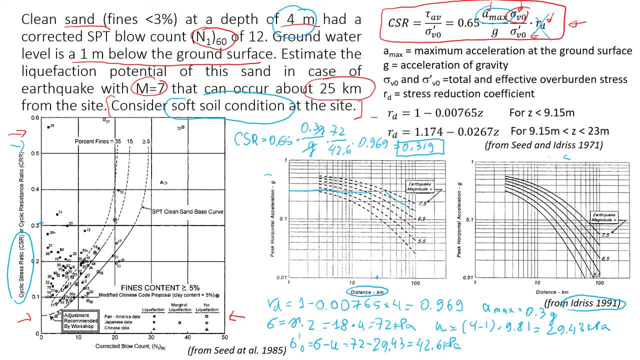 We're going to find our value is about 0.32.. It's here And it's actually pretty high, And we're going to look at the N1.. 60, which is 12.. It's somewhere here, So we have a point here. 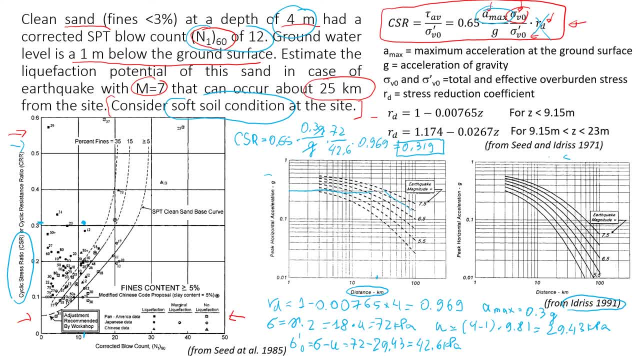 Okay. So the way we look at this chart, You see there's a few lines here. It depends on the percentage of finds. This one is for the clean sand, with percentage less than 5.. So the way we see it, everything in this area is going to liquefied. 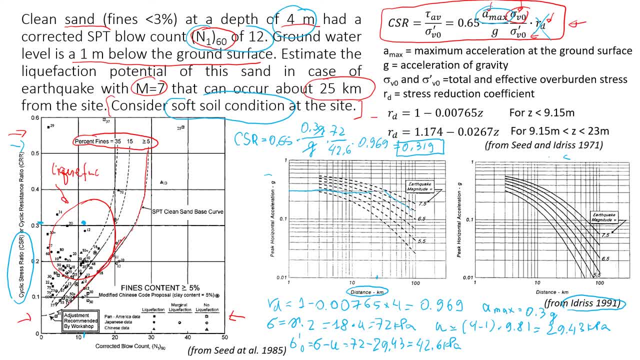 Liquefied, Liquefaction, Everything here there is no liquefaction. So according to our estimates, we have a point in the area where it's supposed to liquefy. So we can say that if there is such an earthquake with a magnitude of 7. 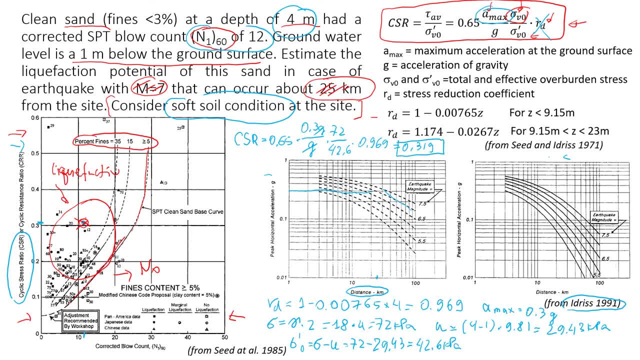 and the epicenter about 25 kilometers from the site, this particular sand will have a high chance to liquefy. Well, that's how we use cyclic stress ratio to estimate the liquefaction potential of sand. Thanks for watching this video. Have a nice day. Bye. 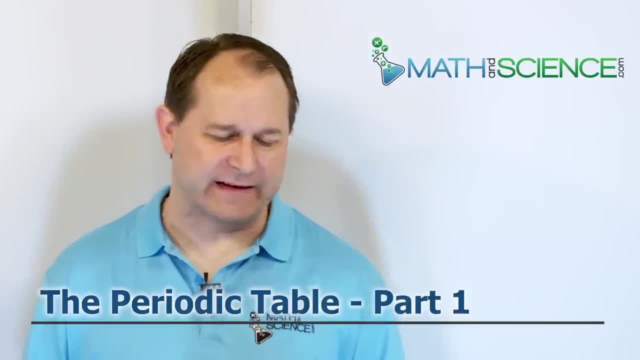 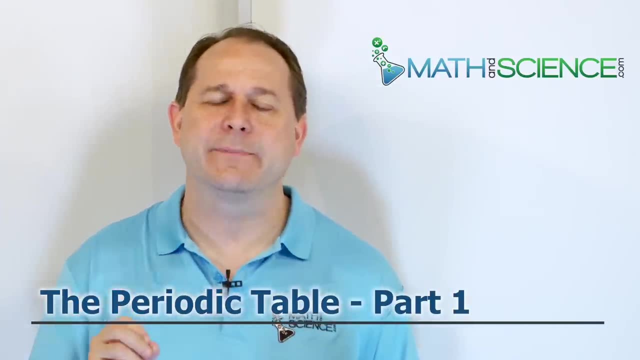 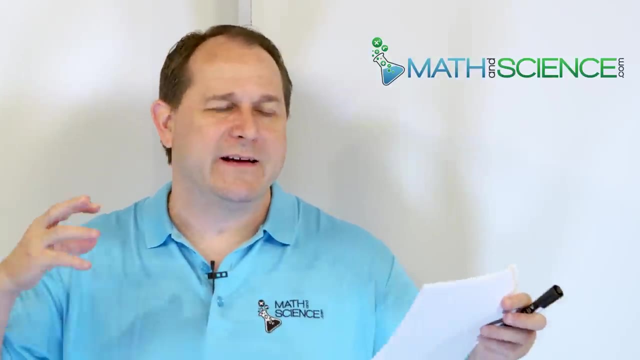 Hello, welcome back. The title of this lesson is called The Periodic Table of the Elements, and this is part one. Now, truthfully, this lesson is one of the absolute most important lessons for anybody who is just starting to learn chemistry, because here we take apart, disassemble. 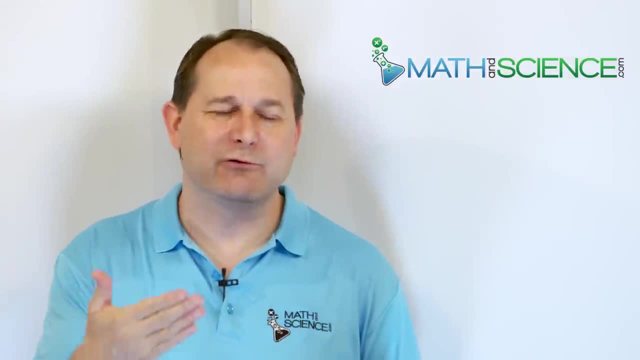 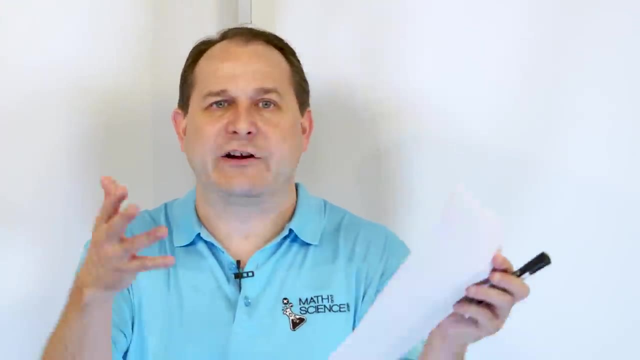 and examine and understand the periodic table, which, literally, is something that you have to become friends with in order to do any chemistry. So in the beginning, when you look at a periodic table, it just looks like a chart with squares on it, But then at the end of this lesson, 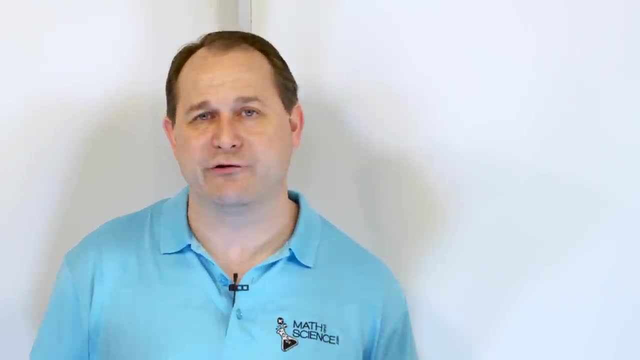 the goal is going to be to take that apart and understand why it's constructed the way it is, what value does it bring, why do we care about it, how do we use it, and a few other things along the way as well. So, without any further ado, let's just talk about this periodic table. 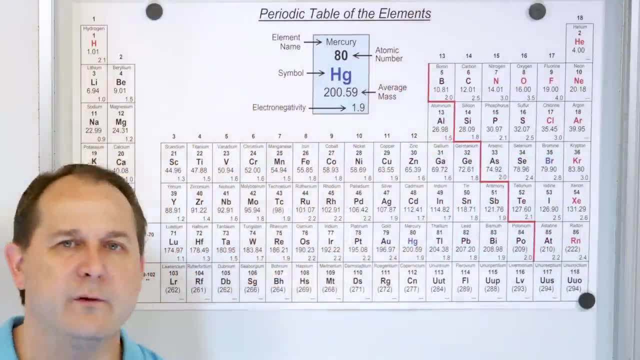 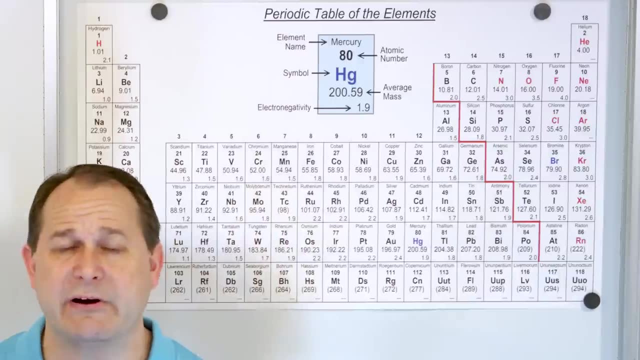 So this is what we call the periodic table of the elements. Whatever textbook you're using, or if you're on the internet or whatever, you can find many different flavors and varieties of the periodic table. So let's get started. So, let's get started. So let's get started. 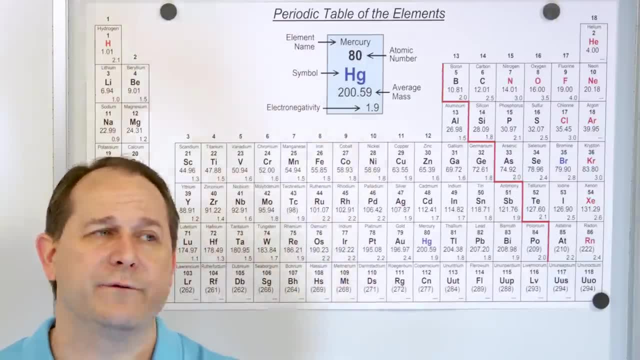 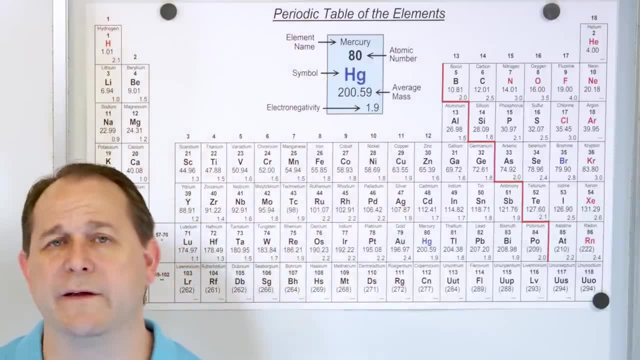 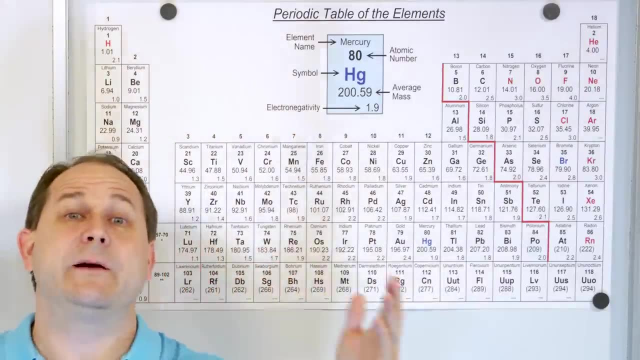 a textbook or whatever. just pull out the one that you have and follow along. They all have a generally the same structure, but of course they'll look a little bit different. All right Now. the big picture of the periodic table is that it contains all of the different.